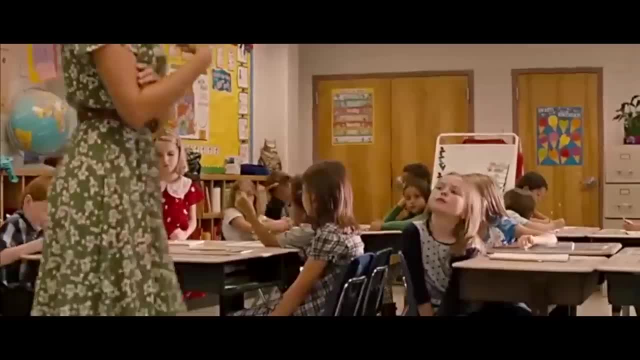 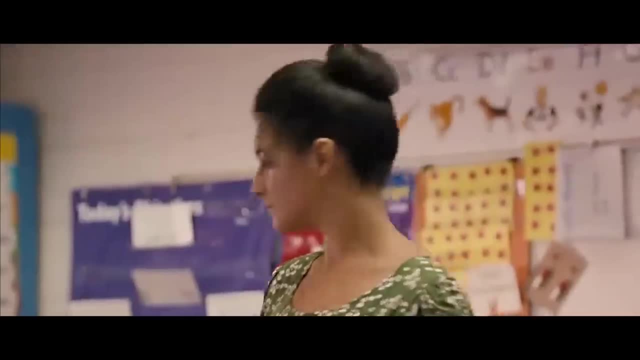 The teacher was relieved to see Mary's embarrassed look, But just as she continued the lesson, the teacher stood around and looked at Sophie. The teacher looked surprised and immediately grabbed a calculator to verify the answer. The teacher's answer was very surprising. Not only did Mary get the result right, 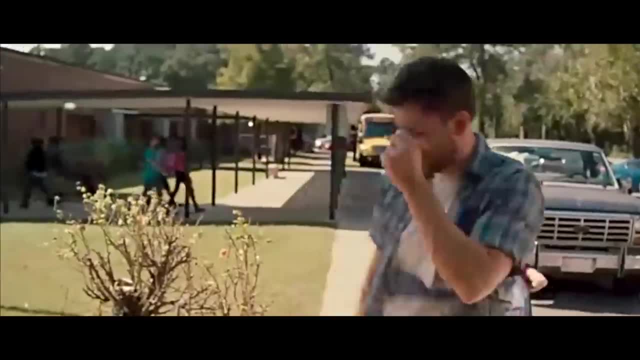 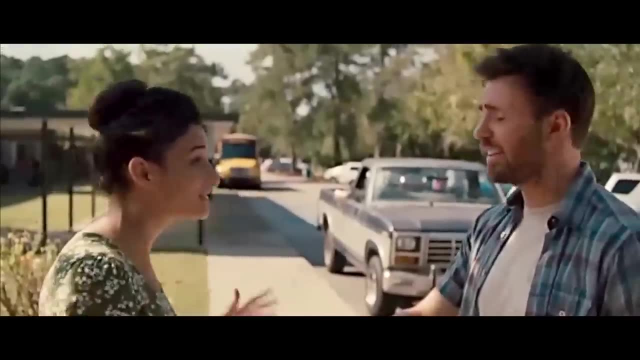 but she even calculated the square root. At the end of the school day, the teacher excitedly told Frank that Mary had a talent in mathematics. Frank, however, acted very calmly and lied that Mary had only learned to do speed calculations and was not the genius she claimed to be. He had a talent in math, for example, The teacher said she was a genius. The teacher said she was a genius because it was something she had learned. And she said she was talented in maths and that she was a very well-trained teacher. 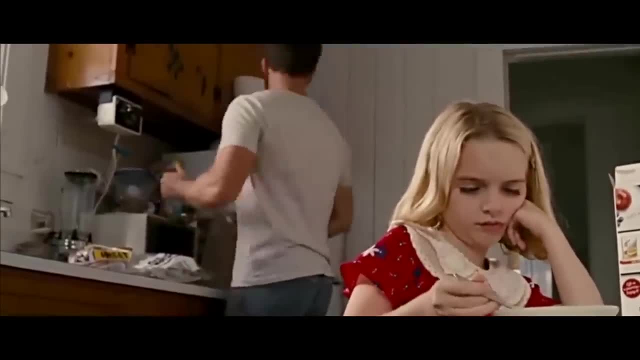 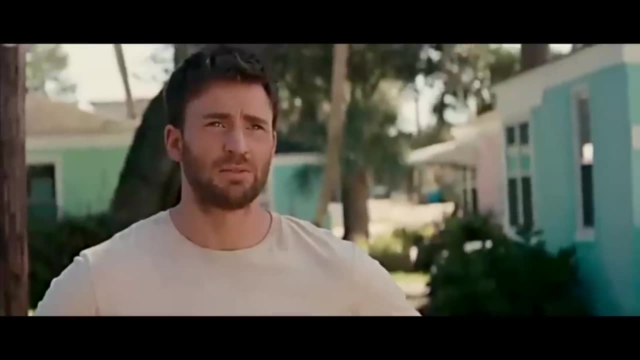 He put his hand on the wall and was at the door with Sophie. The teacher said years ago his sister died by suicide and entrusted him to help take care of Mary, who was only half a year old. In accordance with his sister's wishes, Frank quit his job and moved. 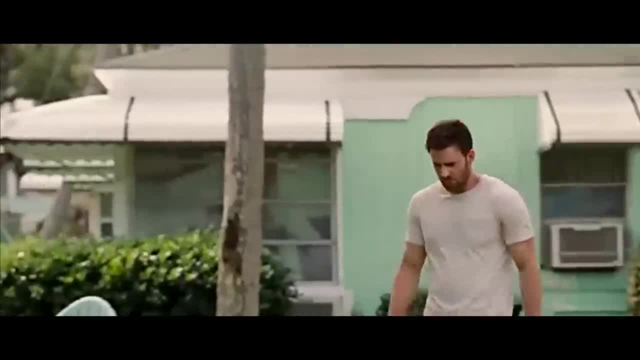 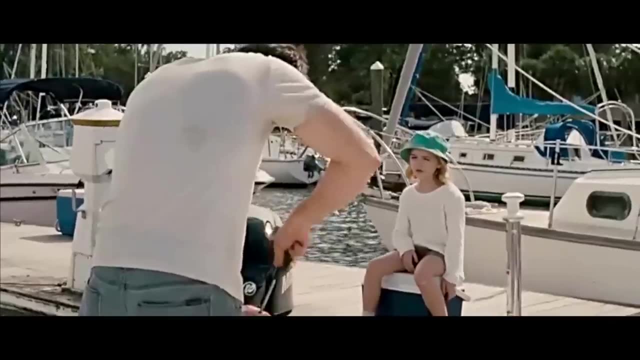 to a small town in the middle of nowhere to live his life as low-key as possible. Mary was naive and kind and adopted a one-eyed yellow cat To make it easier to take care of. Mary Frank works odd jobs at the docks and makes his living by repairing boats. 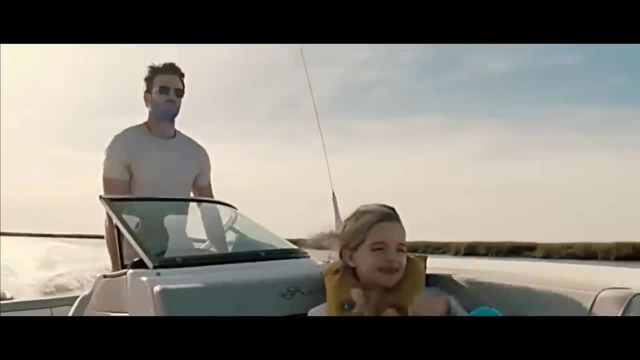 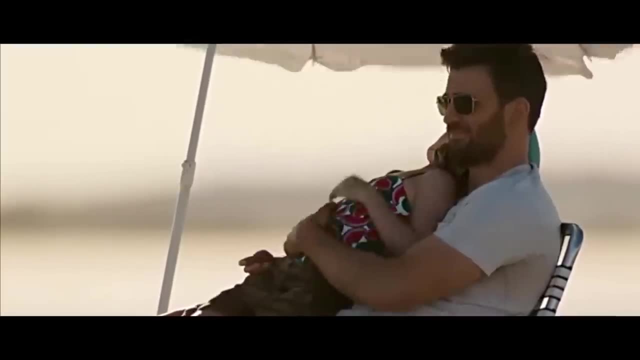 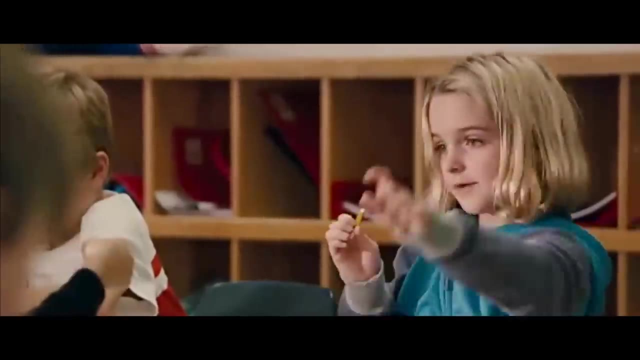 The happiest thing every day is to take Mary out to sea with him, Although life is very poor, but watch Mary grow up day by day. Frank felt a kind of happiness that he had never felt before When Mary started school. all kinds of trouble followed, and the elementary school curriculum. 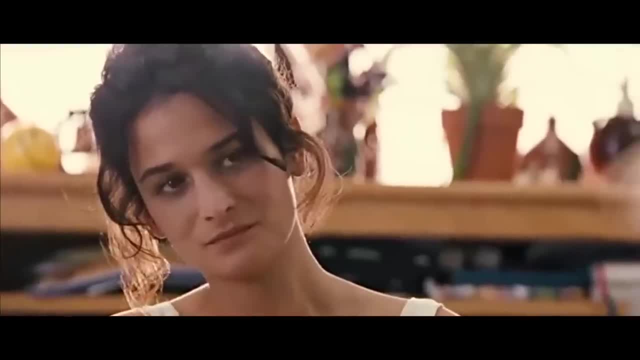 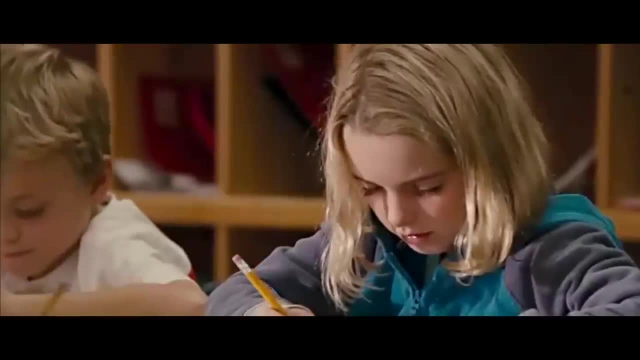 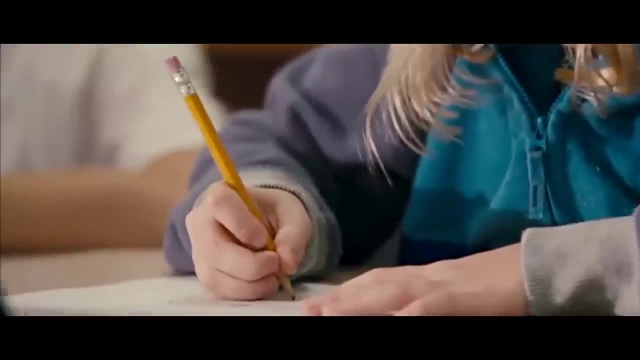 was no challenge at all for Mary. Ms Susan prepared herself by taking out a high school math paper and giving her a test. Mary looked at the questions with interest, picked up a pen and began to answer them. The teacher was looking forward to it and after only 15 minutes Mary finished the test with a. 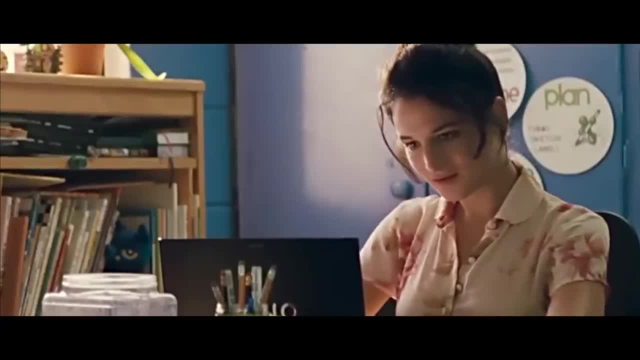 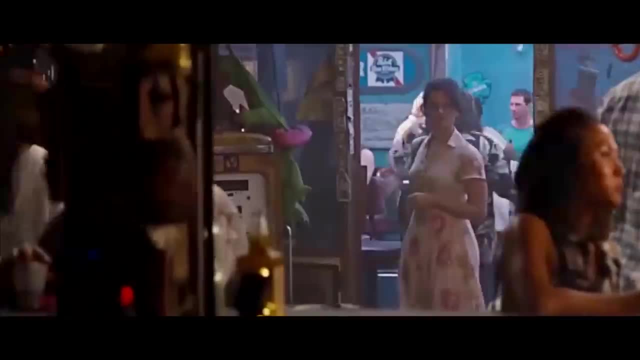 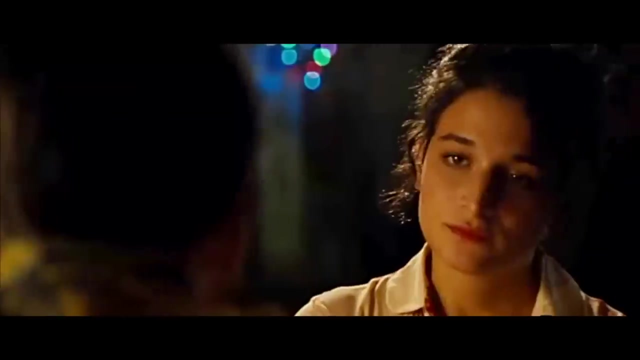 perfect score. Ms Susan was even more convinced that Mary was a genius. Susan couldn't understand why Frank would overlook Mary's talent. That night she went into the bar where she had never been before and found Frank to understand the situation. During the conversation, Susan learns: 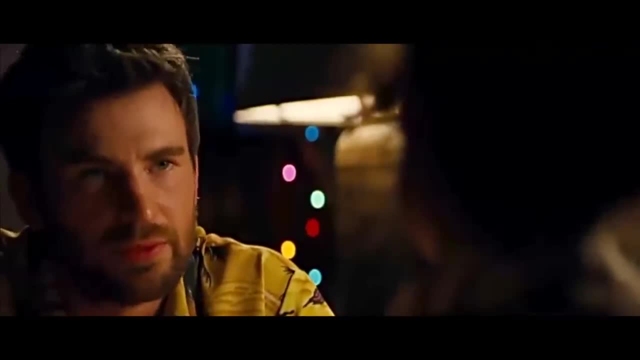 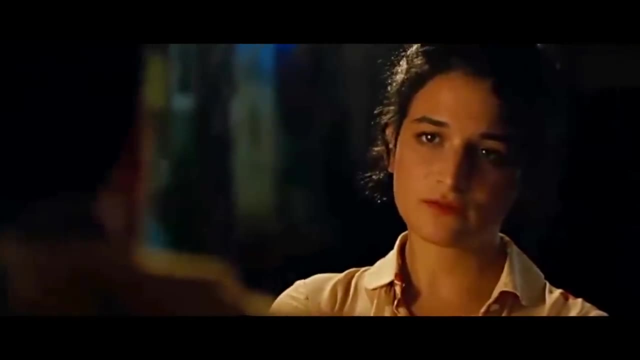 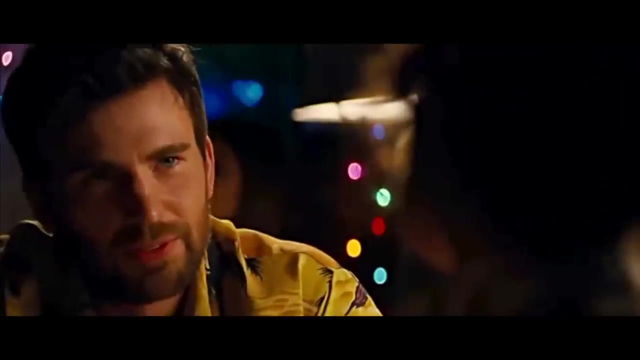 that Mary's mother, Diane, was also a rare mathematical genius who, under the pressure of her mother, Anna, had been solving all kinds of mathematical puzzles since childhood and eventually chose to commit suicide because she was overwhelmed. She entrusted Mary to himself because she did not want to see her child repeat the same life as hers. But gold always shines. 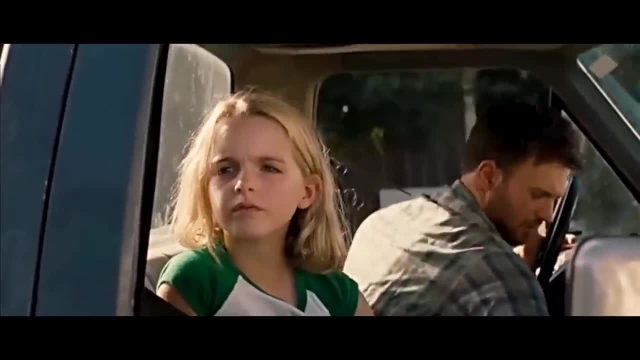 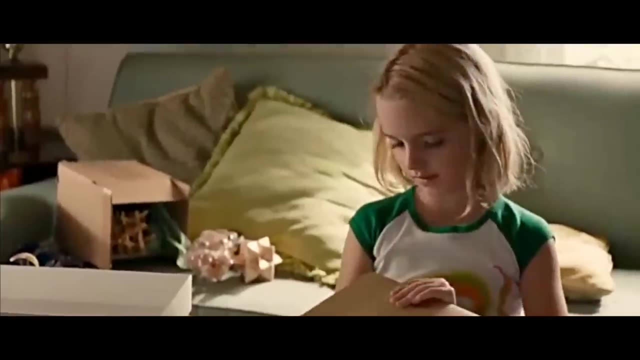 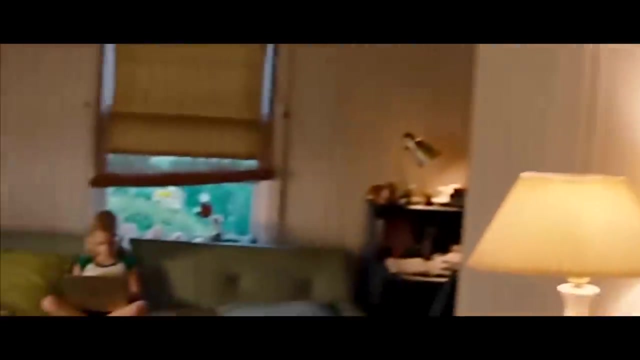 and Mary's talent can't be hidden. A few days later, Frank's worst fears came true. Grandma Anna found them after learning the news. She gave Mary a laptop filled with various math lessons, and the purpose of doing so was obvious enough. Watching Mary's full attention: Frank 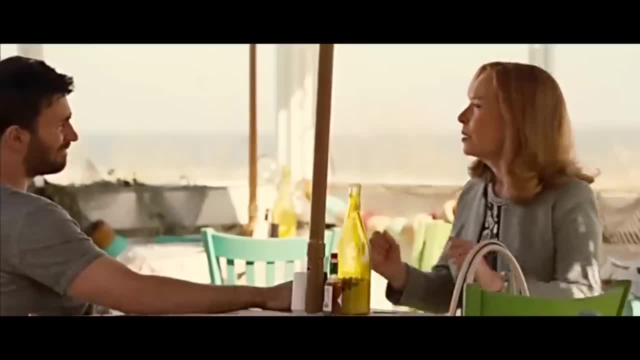 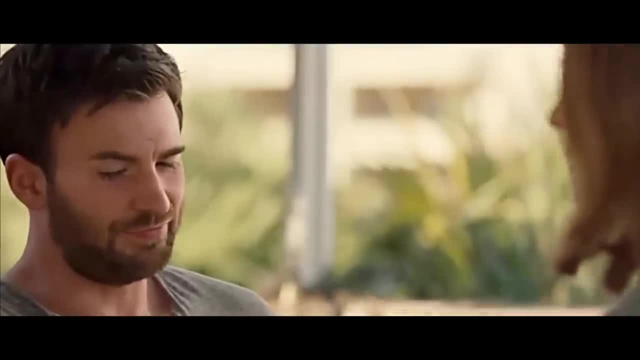 couldn't help but be nervous. Anna didn't care about her son, and she used her position and power directly to force Frank to give up custody. It was clear from this that the death of her sister Diane did not make Anna change anything. Frank also did not give in and insisted on keeping. 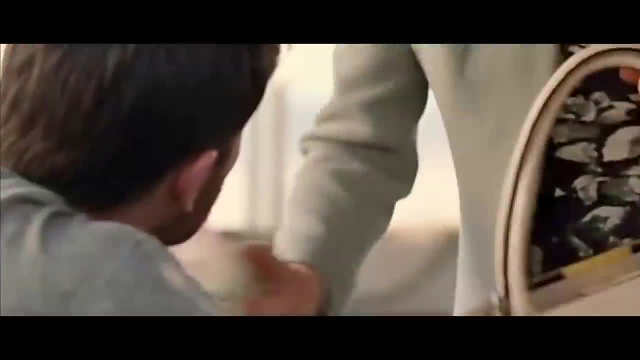 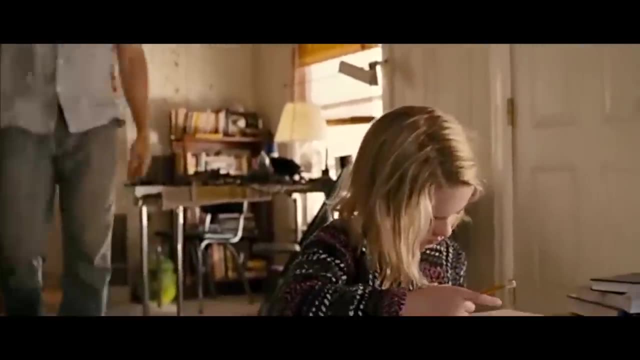 the child with him and the first negotiation between them- this kind of- fell out. unhappily, Because of more and more of this, Frank's mother, Diane, and her son Frank were all in the same situation, With more math classes. Mary is obsessed with her studies and loses interest. 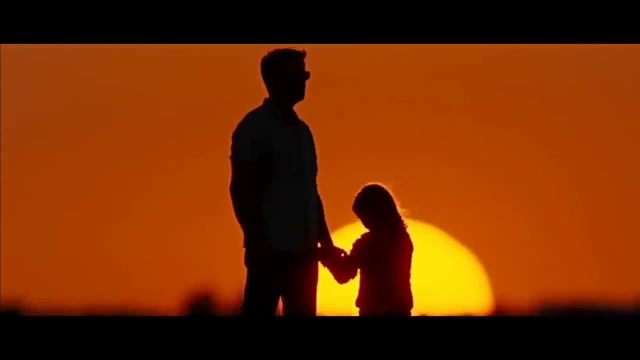 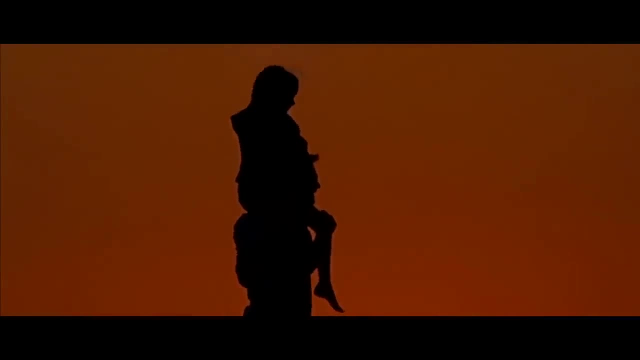 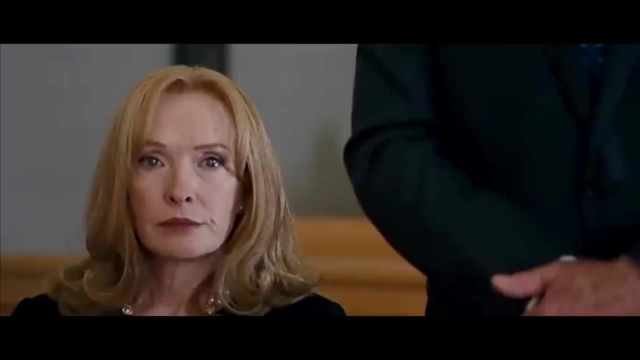 in everything outside. Frank was anxious, ie afraid of losing Mary, but also worried that it would ruin her life. After a struggle, he decided to keep custody. Anna soon filed a lawsuit in court. Frank could not afford a fancy lawyer. The opposing lawyer, who is experienced, accused 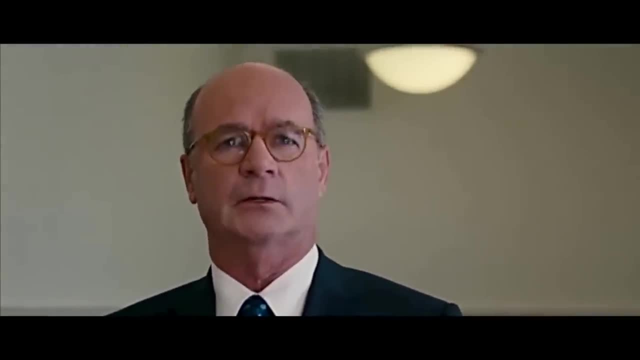 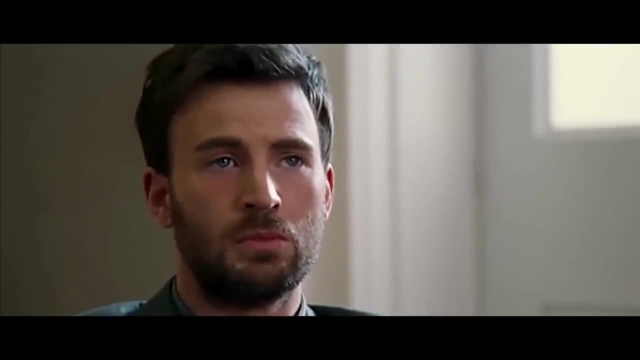 Frank of illegally occupying custody and making Mary live in a bad environment. Frank's lawyer, Diane, argued that Frank had adopted Mary in full compliance with his sister's will and that there was no legal problem at all. As for what they said about the poor living environment after his 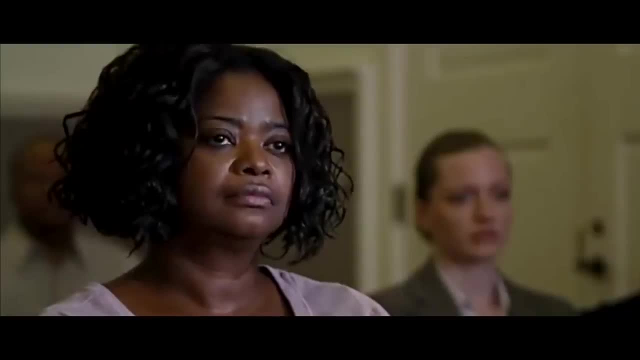 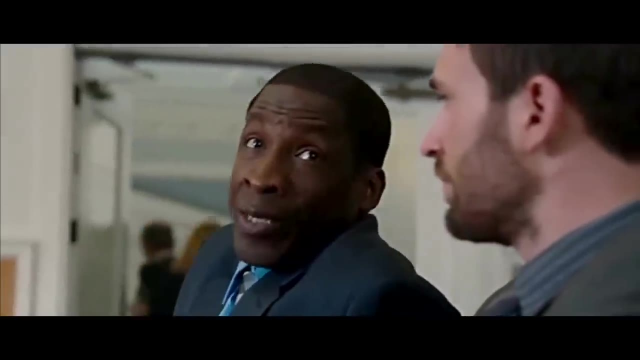 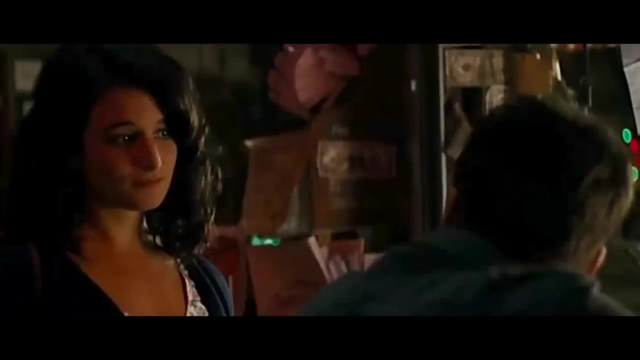 on-the-spot investigation, he thought that the other side was nonsense. In the end, Anna was only granted visitation rights to Mary, which made Frank breathe a sigh of relief That night. while Mary is spending the night at a neighbor's house, Frank comes to the bar to relax and happens to. 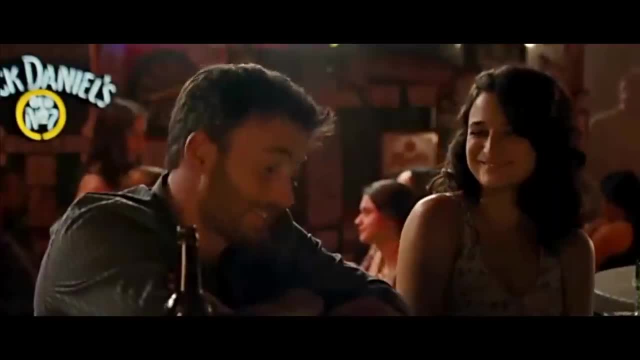 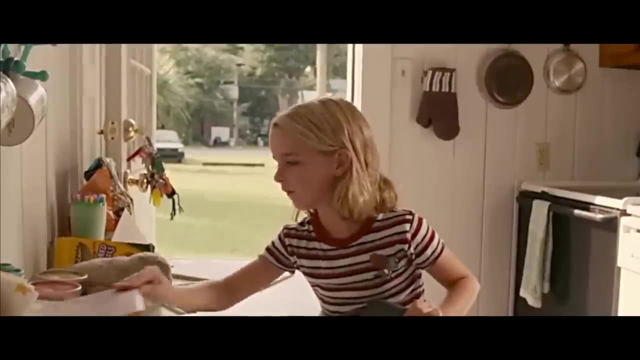 meet Miss Sophie and the two have a good time. Frank's mother, Diane, argued that Anna was having a good time drinking and talking Under the influence of alcohol. their relationship is closer. Early the next morning Mary came home to get her things and saw Sophie who had just 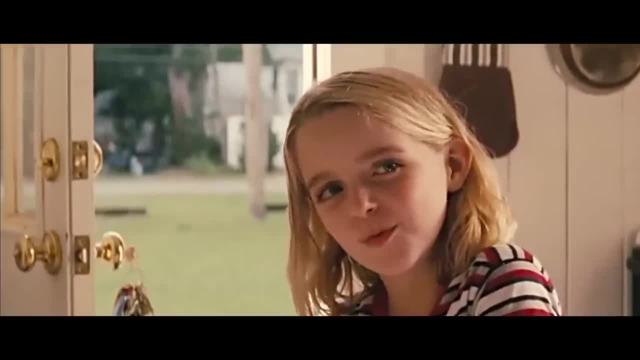 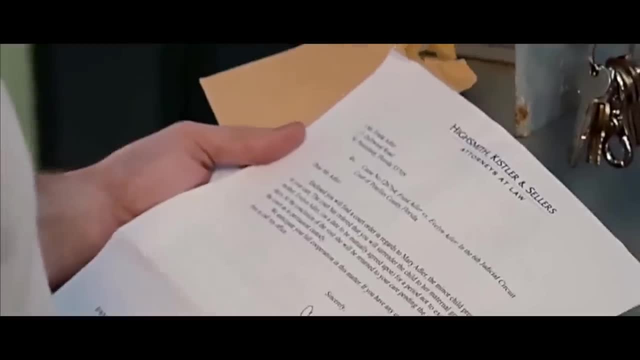 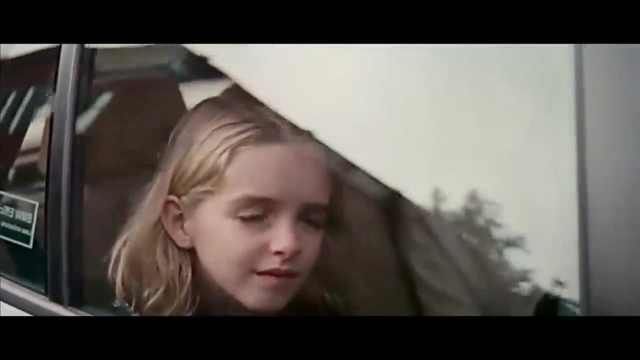 woken up. Mary is only seven years old, but she knows her uncle very well. For a moment, Miss Sophie was extremely embarrassed. That afternoon Frank received notice from the court that Anna was taking Mary with her on a two-day vacation to Boston. It is the first time Mary leaves town. 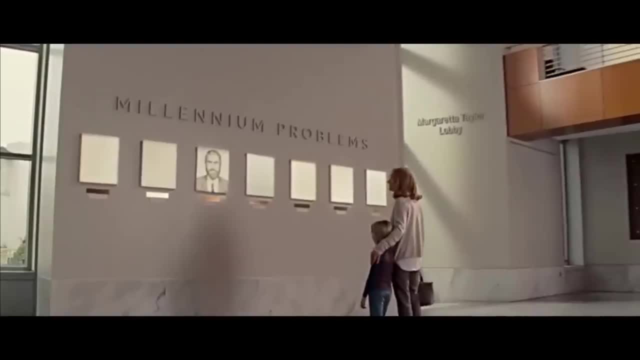 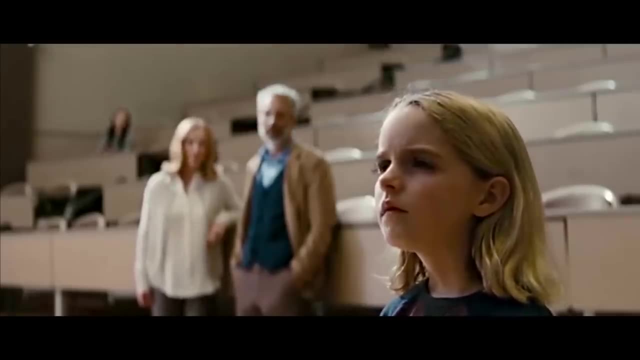 and the first time she sees a picture of her mother. The next day, Anna takes Mary to Boston University, where a professor has prepared special questions to test her mathematical talent. However, Mary looks at the questions and never acts, and the professor looks disappointed that. 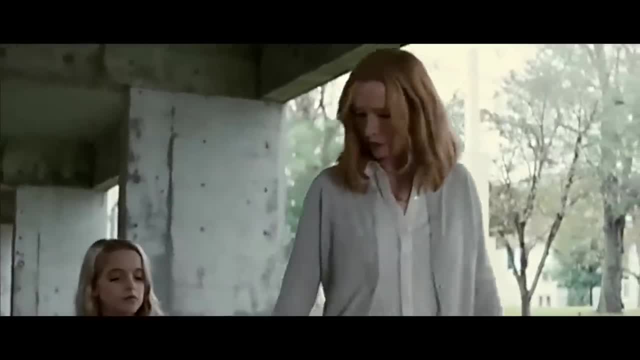 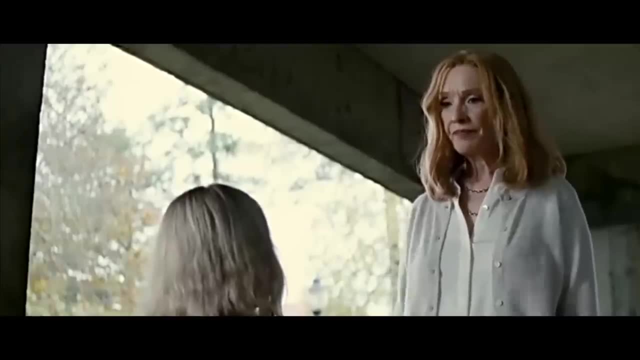 Mary cannot answer them. Just as the two are about to leave, Mary tells Anna that the professor's problem is missing a symbol and cannot be reasoned with. Anna immediately takes her back and when the problem is clear, Mary picks up the question and says: 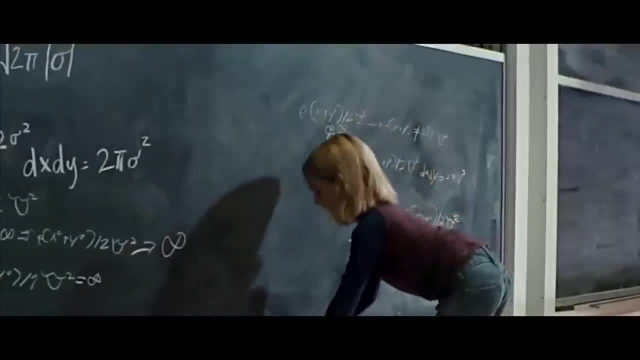 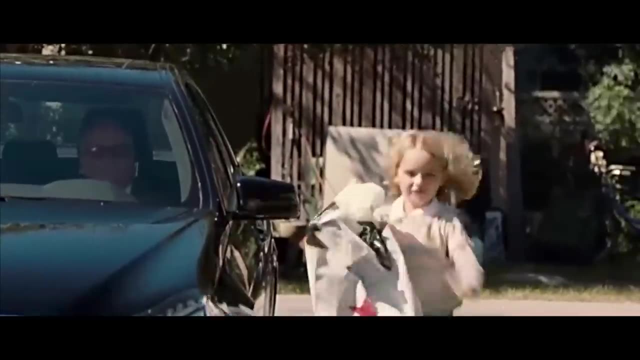 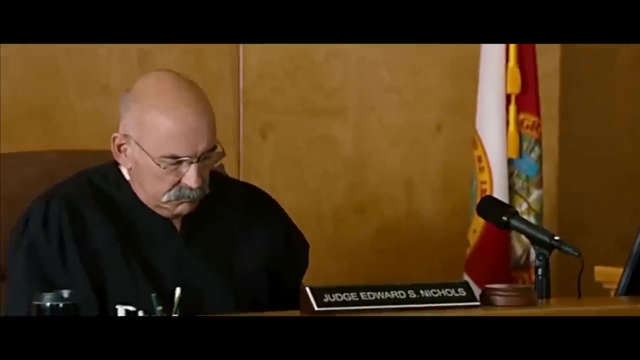 Anna picks up the chalk and begins to perform the calculations, which are written all over the two blackboards, arriving at a quick and accurate conclusion. The two-day journey was soon over. Anna has made up her mind to keep Mary by her side. The court was soon in session for a second. 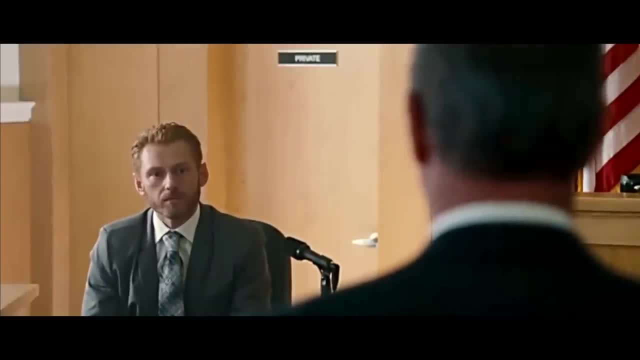 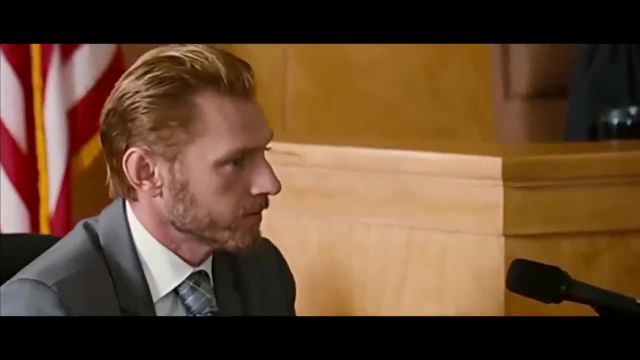 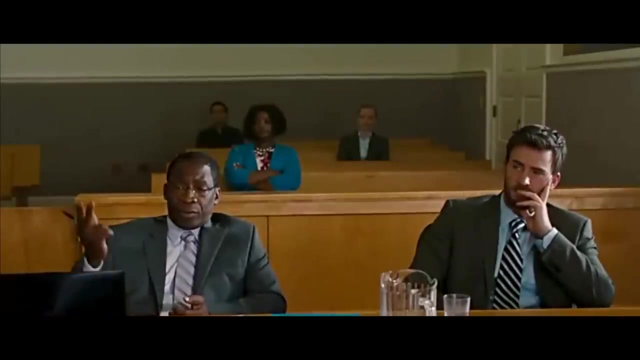 time. This time, Anna brought in Mary's biological father. The man falsely claimed that he had searched for the child after Diane's death. as the child's father, he was willing to let Anna become a legal guardian. Seeing that the situation was not good, the lawyer was calm in the face of danger. 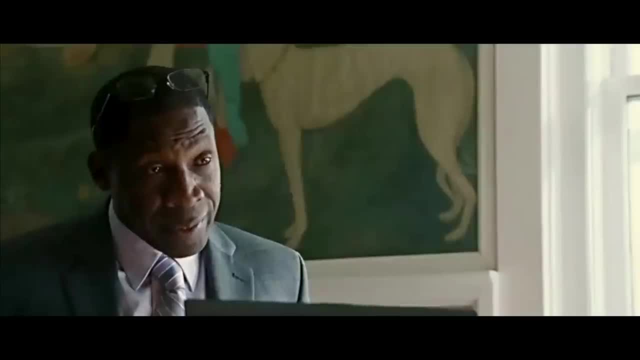 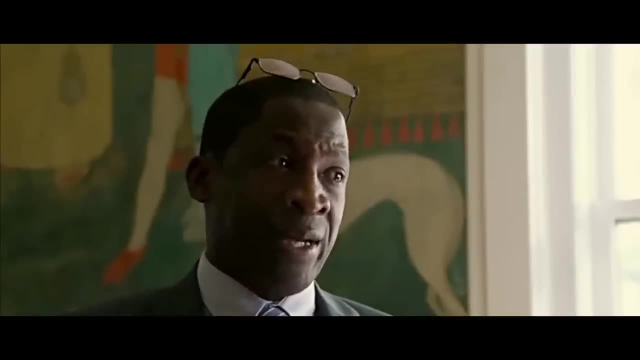 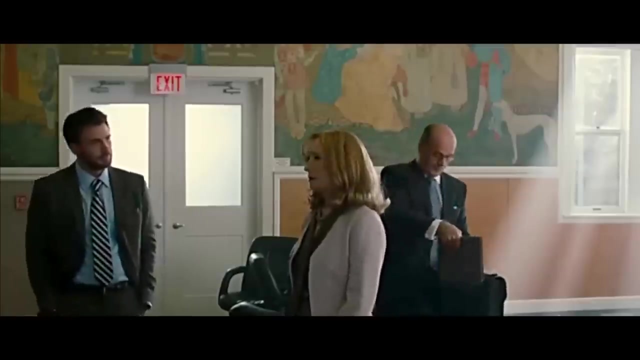 and questioned the man who had never seen Mary- even Mary's full name was not clear- and had not fulfilled his father's responsibilities at all. Even if he was the father of the child, he had no right to appoint a guardian. A brilliant defense was supported by the judge and, once again, Frank 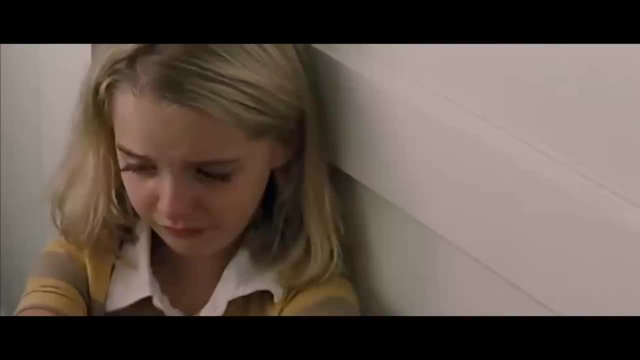 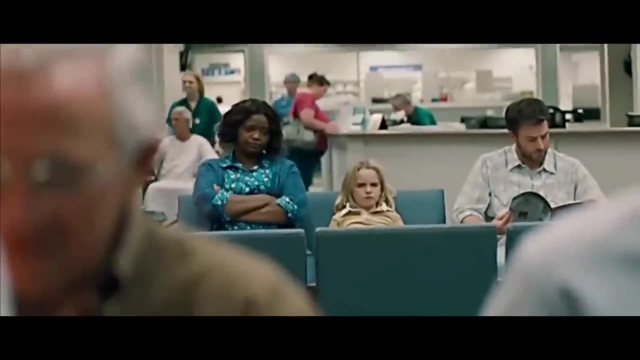 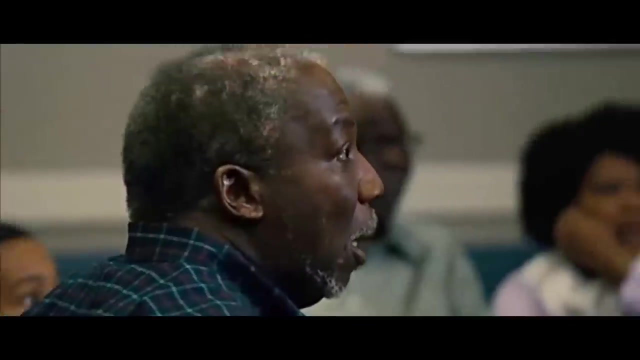 prevailed retaining custody for the time being, But Mary heard that her father wasn't even going to visit her And hid in her room crying with sadness. In order to heal Mary's broken heart, Frank took her to the hospital and waited quietly in front of the maternity ward When the baby's cry came from. 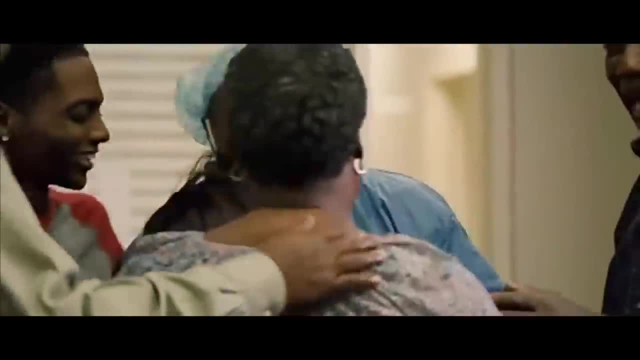 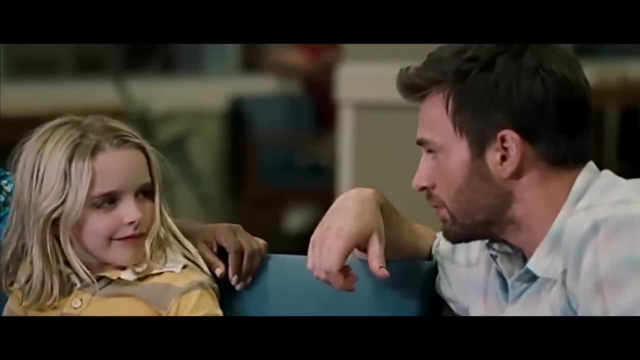 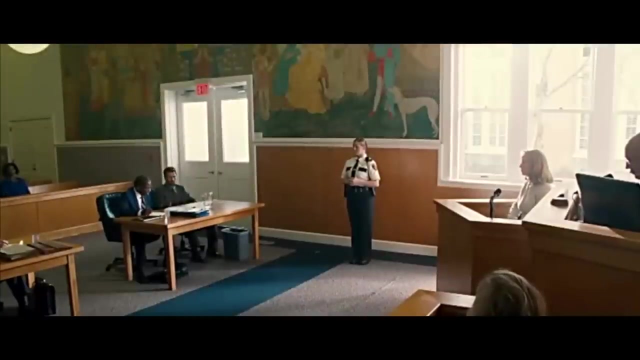 the delivery room. the family waiting anxiously outside the door cheered. This scene moved Mary deeply. Frank told her I was just as happy as they were when you were born. I will always be with you, no matter when or where you are. A week later, the court sat for a third time. 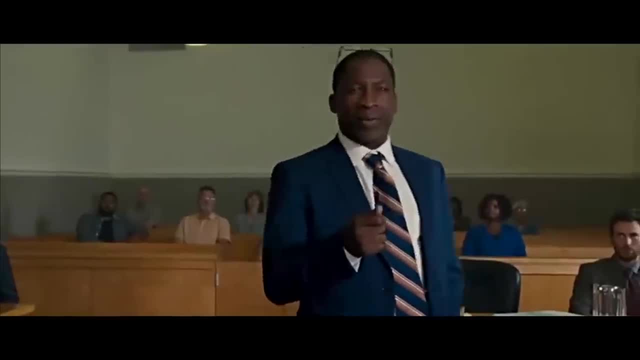 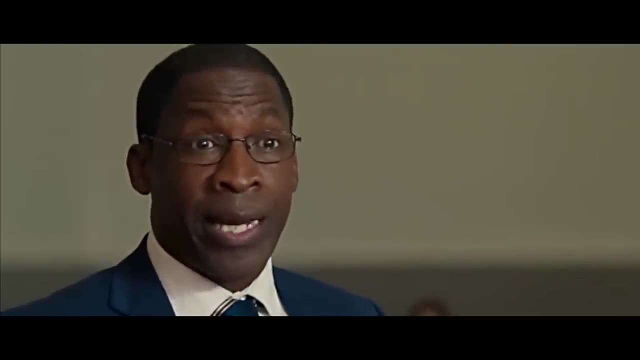 Based on a detailed investigation. the attorney claimed that Anna's control over Diane's life and the imposition of her personal will on her was a key factor in Diane's suicide. Anna instantly lost control and became hysterical in the courtroom, and the opposing attorney did. 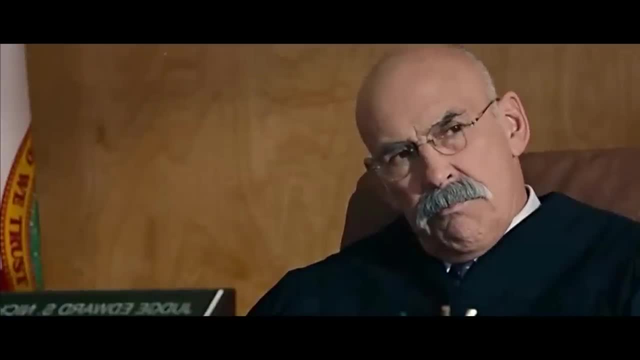 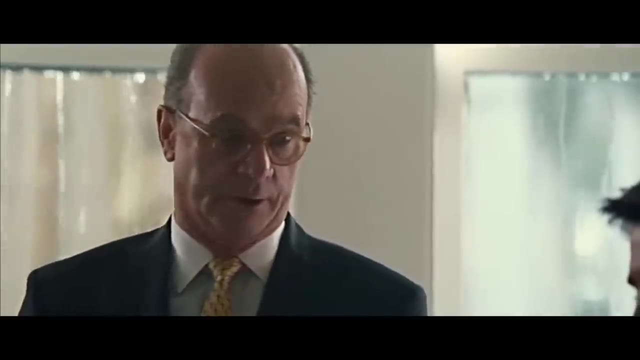 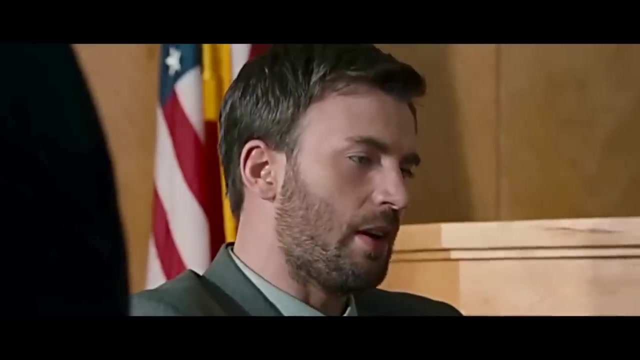 not relent claiming that Frank had no formal job or health insurance and had difficulty providing quality resources in terms of education and medical care. Not only that, but Frank had a history of fighting and brawling, Not ruling out his propensity for violence. The barrage of questions was like a sharp knife. 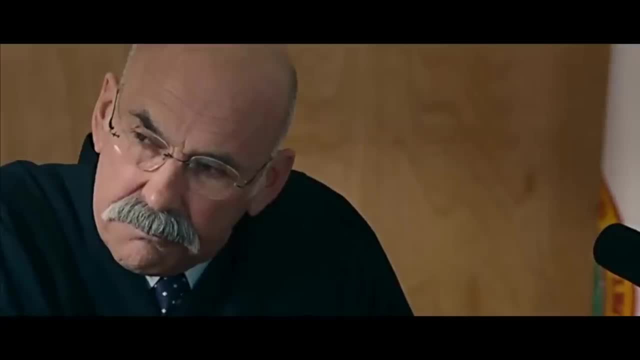 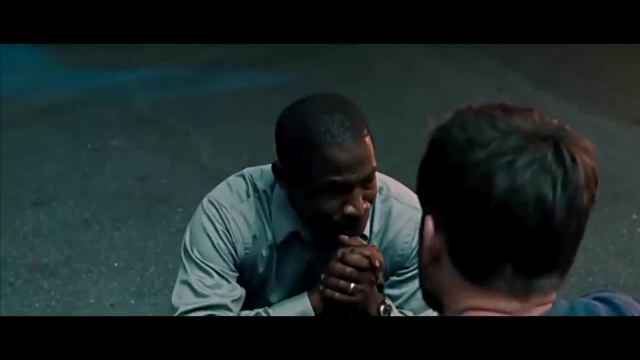 each one poking at Frank's vitals. As the arguments came to an end, the court finally chose to adjourn again. That evening, the lawyer approached Frank and told him that, based on his years of knowing the judge, they were likely to lose the case, and it would. 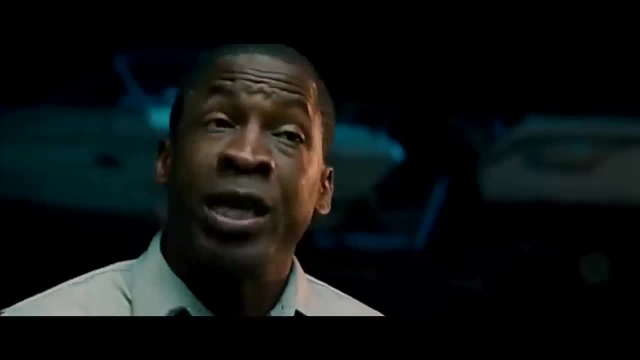 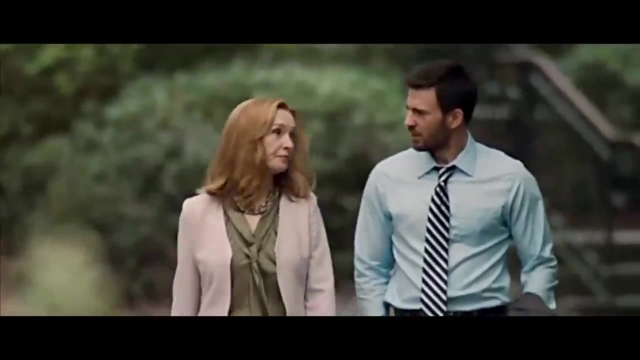 be best to settle out of court before the court made a final decision. After a long night, Frank finally succumbed to reality. Anna proposed that both parties should be released from the court. Frank and the other parties relinquish custody and find a quality foster home nearby, which would 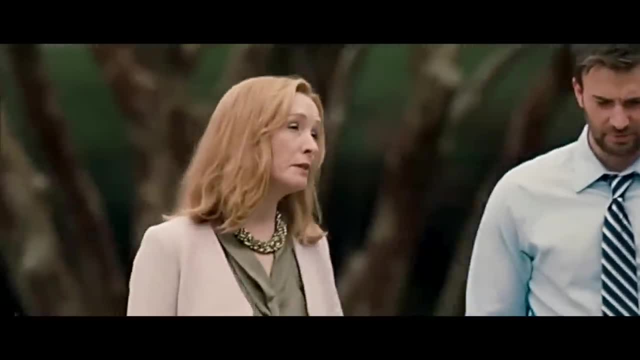 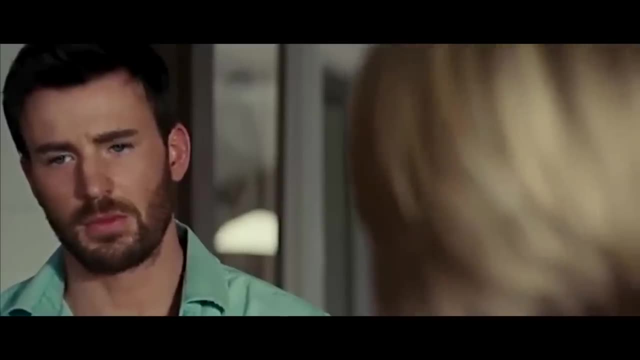 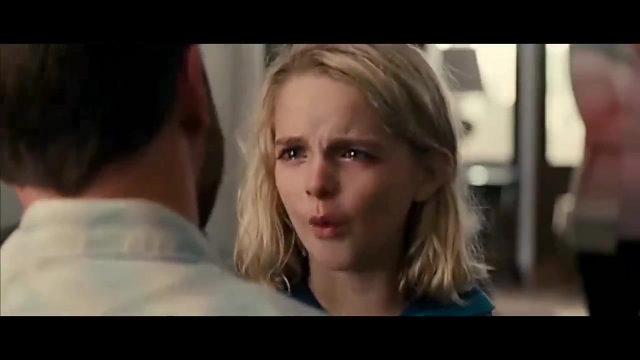 ensure that he could see Mary at all times and allow Mary to avoid Diane's tragedy. He arrived at the foster home with a smile on his face, carefully surveying their home environment and informing them of Mary's habits. The day of separation soon arrives and Mary cries so hard. 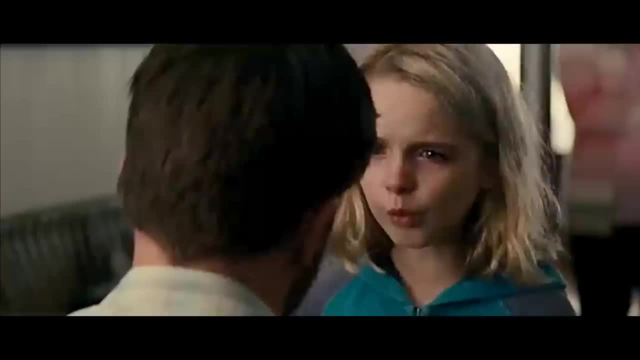 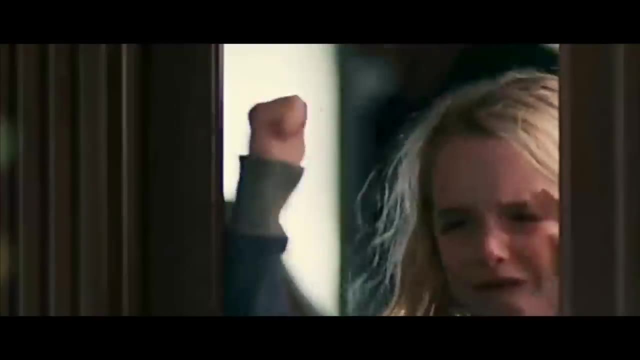 that she loudly rebukes Frank for betraying her and leaving her alone. Looking at Mary's sad face, Frank could not bear to look at her. Frank, who had been with her for so long, could not look any longer and got up to leave. Mary was left to shout incessantly, But it was too. 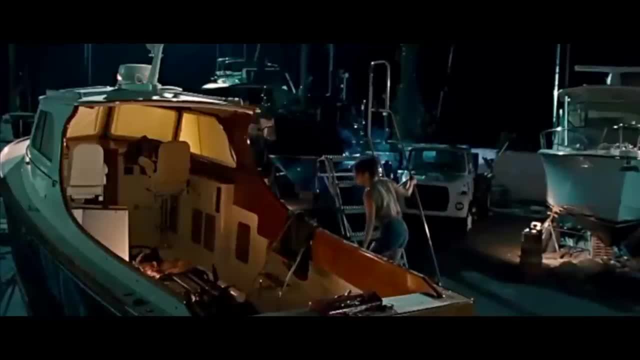 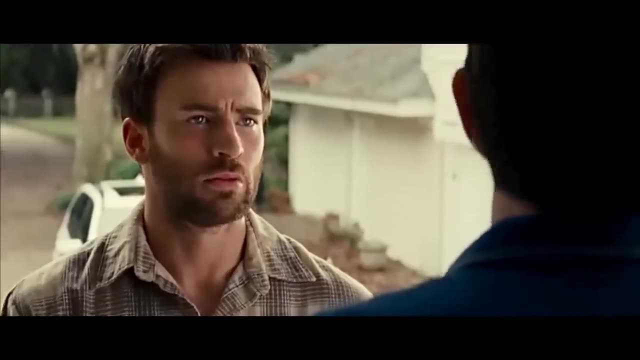 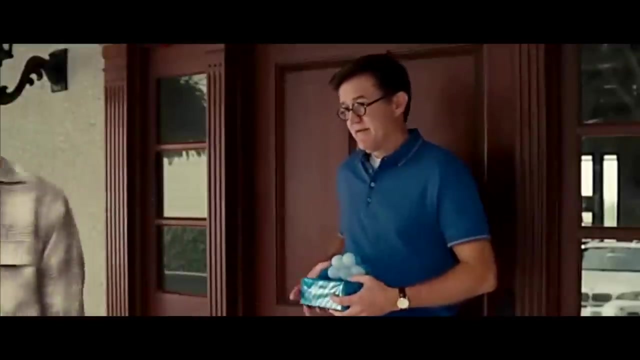 late Frank began to torment himself with work frantically. he wanted to wait for Mary to calm down and then bring a gift to visit. But to his surprise the man stopped him at the door and said that Mary never wanted to see him again. Frank has no choice but to leave the gift and leave. 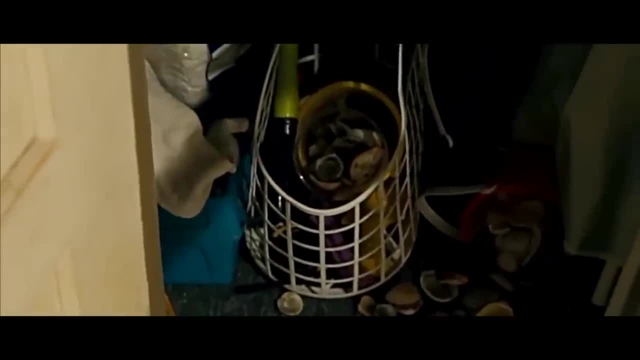 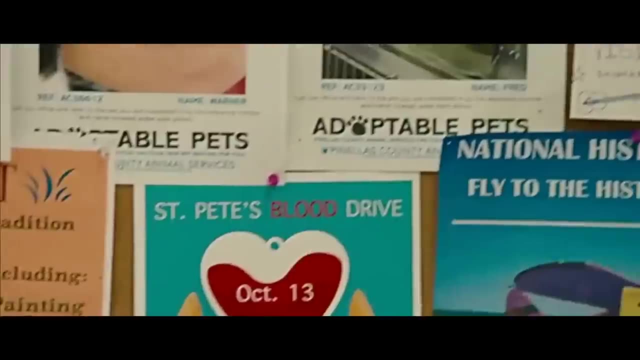 Back home Frank sulked every day and could only look at Mary's toys and miss her. Until that day, everything changed. On the bulletin board in the library, Miss Sophie saw Mary's one-eyed cat being displayed on it by the pet shelter.